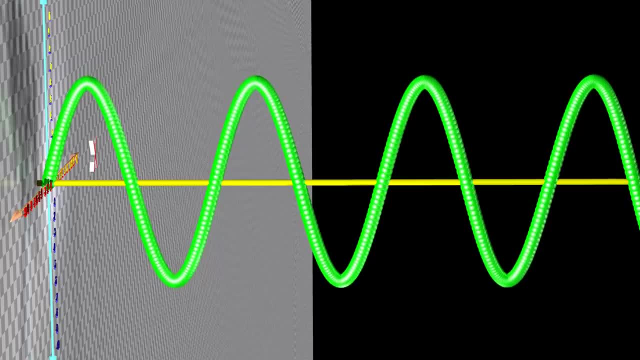 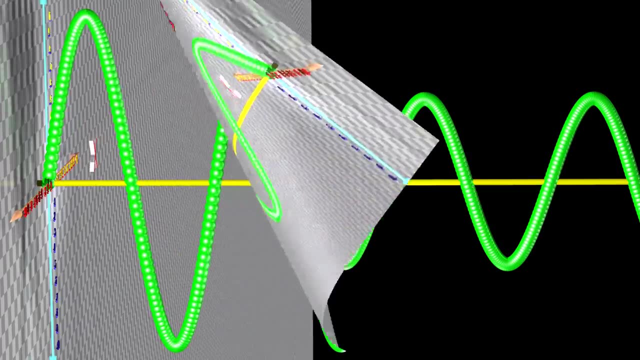 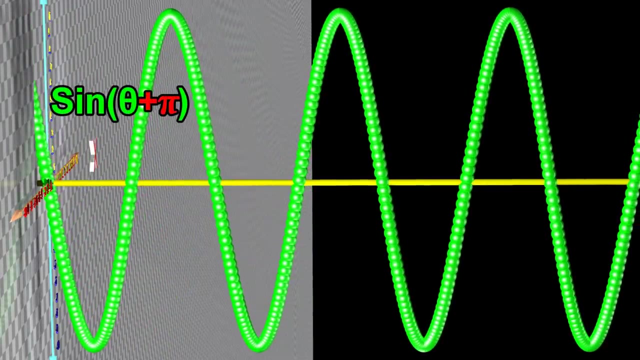 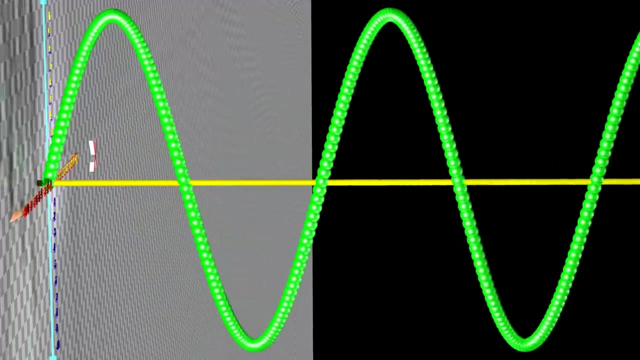 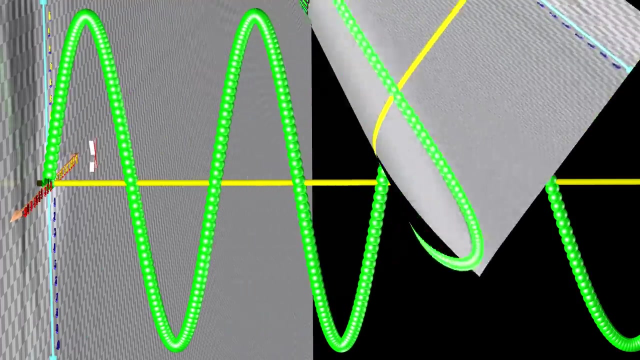 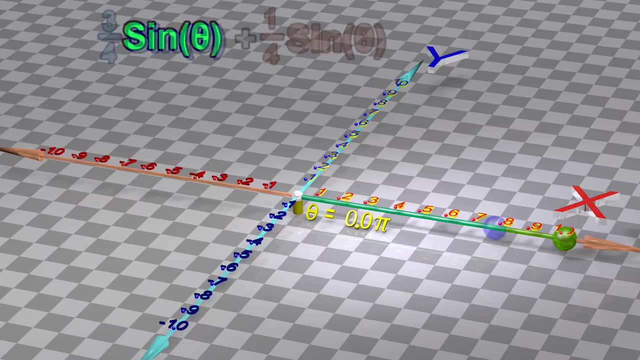 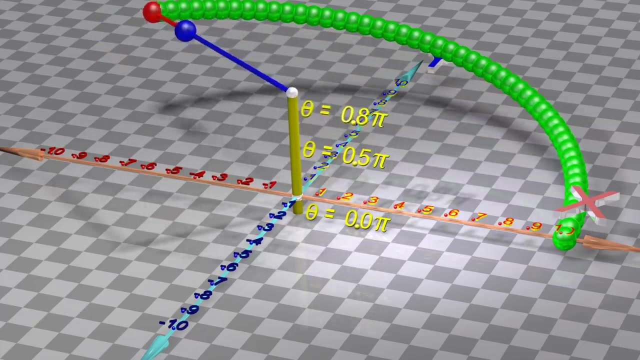 We can change the sine wave's amplitude, phase and frequency. Suppose we have two sine waves that are identical except for the fact that they have different amplitudes. If we add these two sine waves together, the result can be represented graphically as shown. 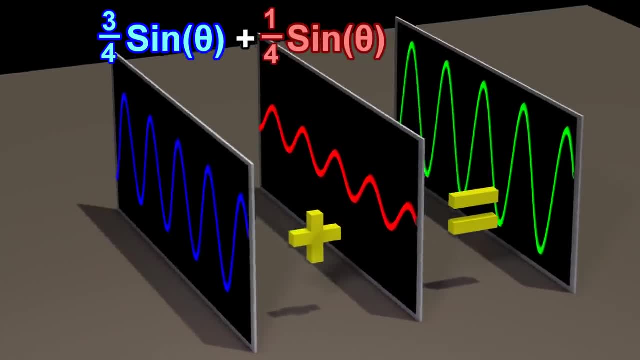 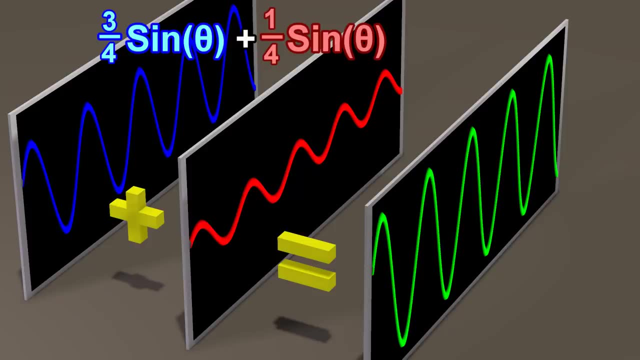 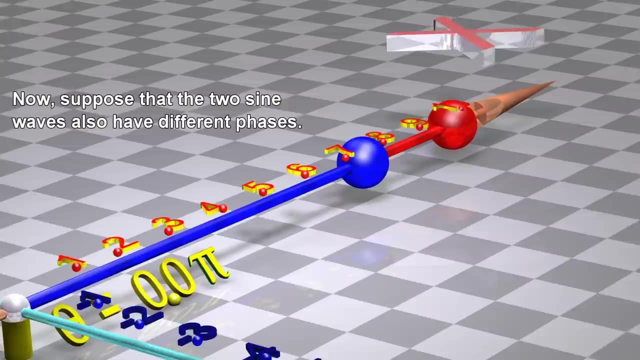 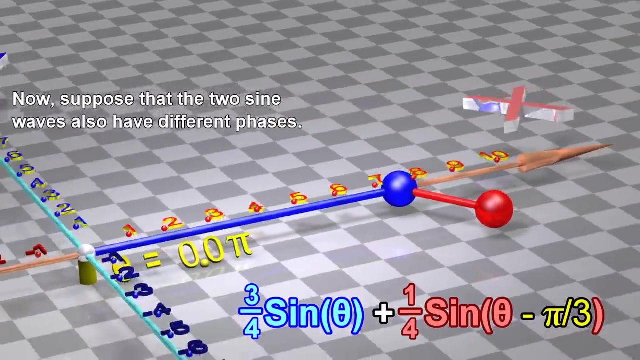 Since the two sine waves are identical, the wave will be equal. Therefore, if x goes higher than the y-axis, the y-axis will be greater than the y-axis. Now suppose that the two sine waves also have different phases. The sum of these two waveforms? 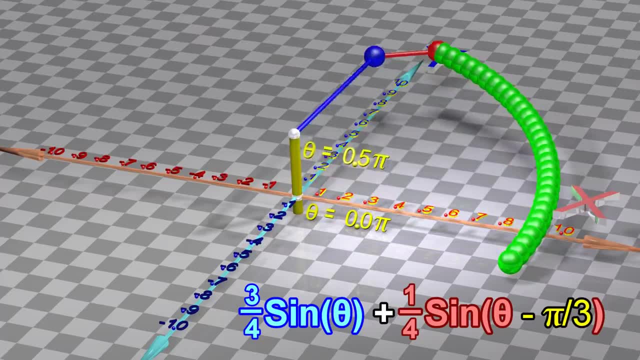 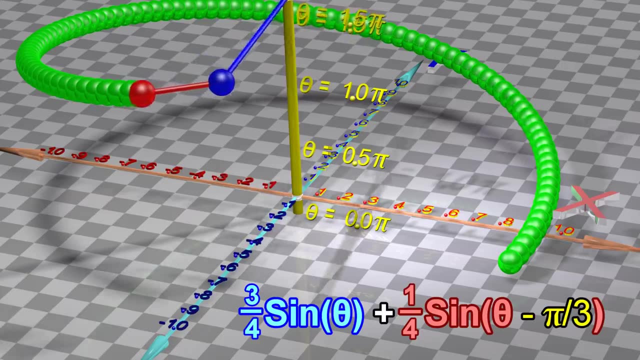 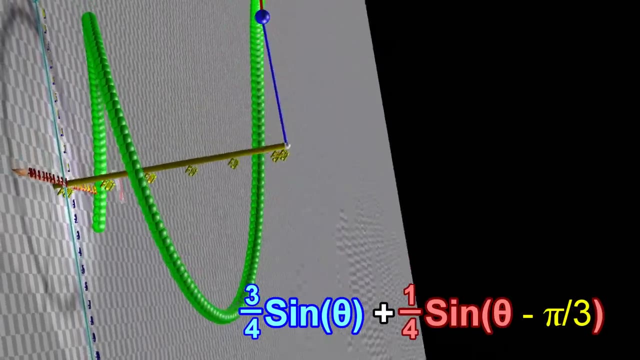 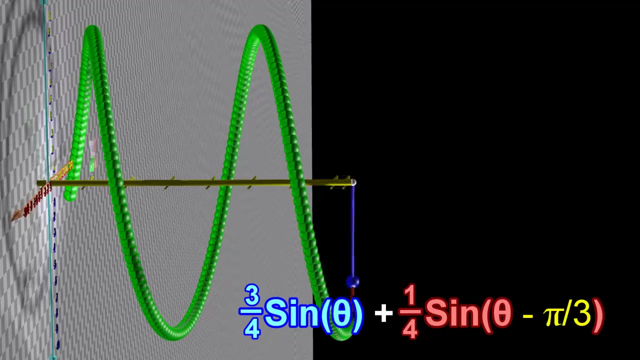 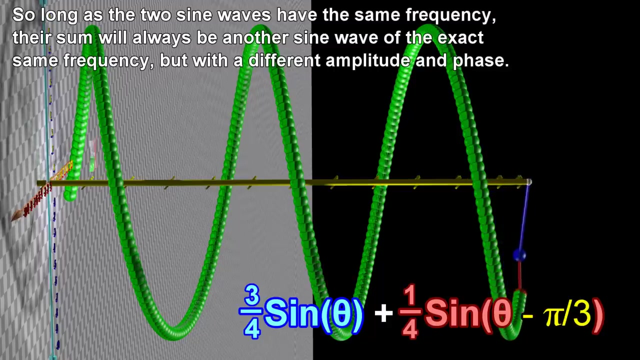 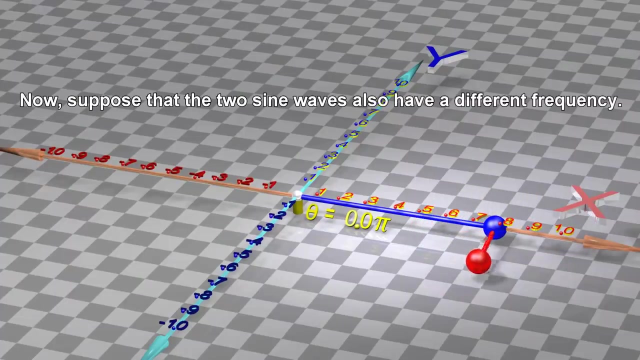 Waveforms can be represented graphically like this: So long as the two sine waves have the same frequency, their sum will always be another sine wave of the exact same frequency, but with a different amplitude and phase. Now suppose that the two sine waves also have a different frequency. 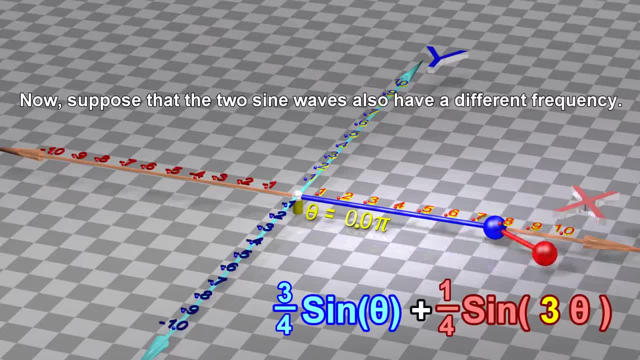 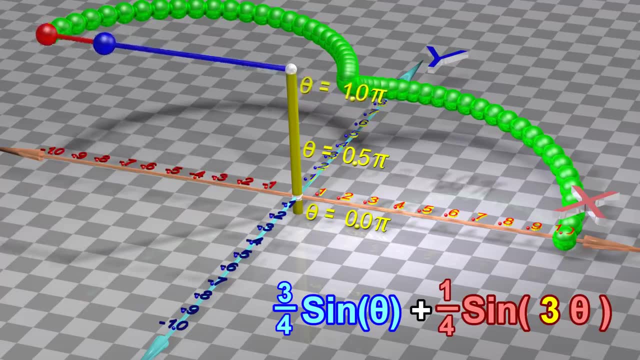 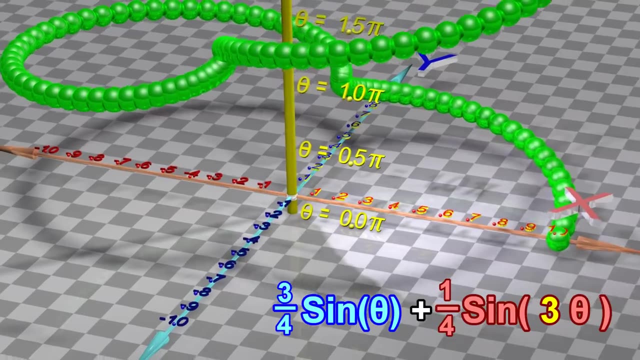 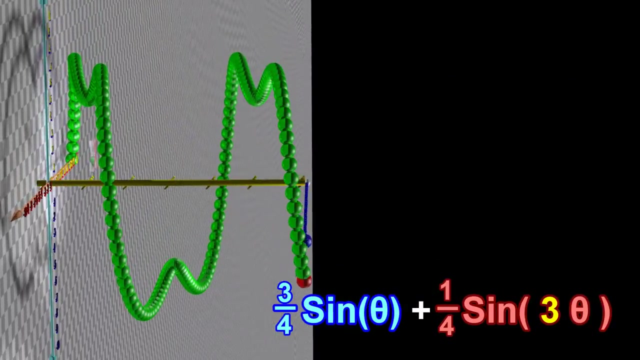 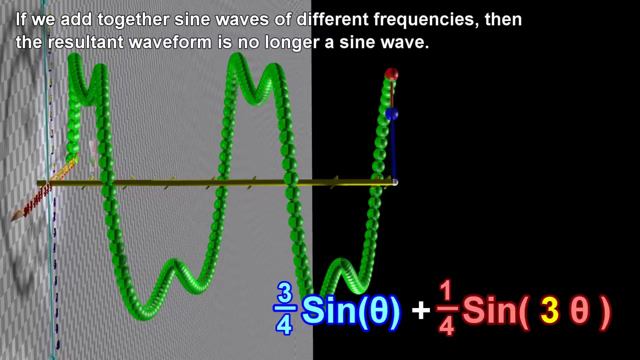 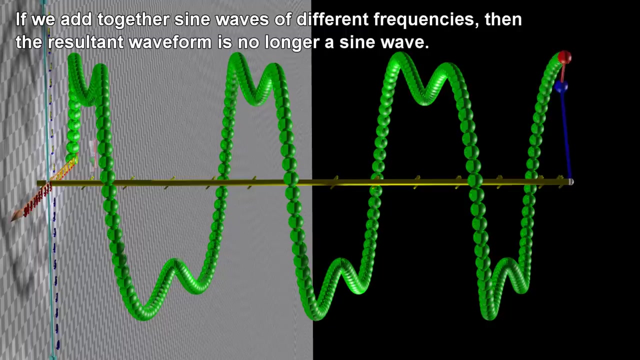 If we add together sine waves of different frequencies, then the resultant waveform is no longer a sine wave. However, the outcome is a sine wave, but the output voltage is one sine wave If we look at this straight line via the fightingaw lugares. 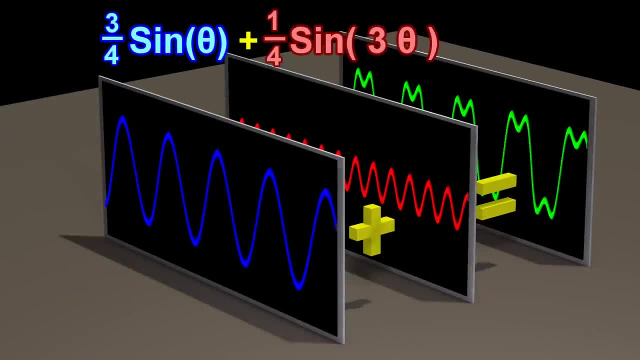 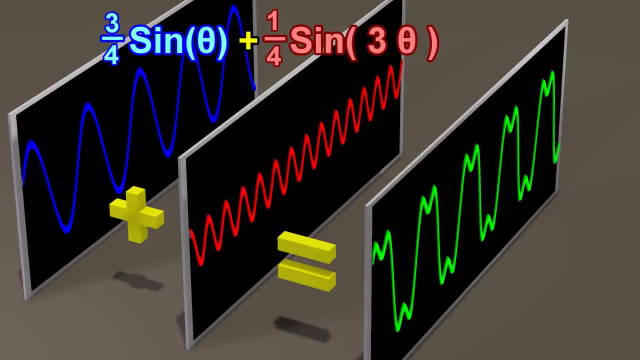 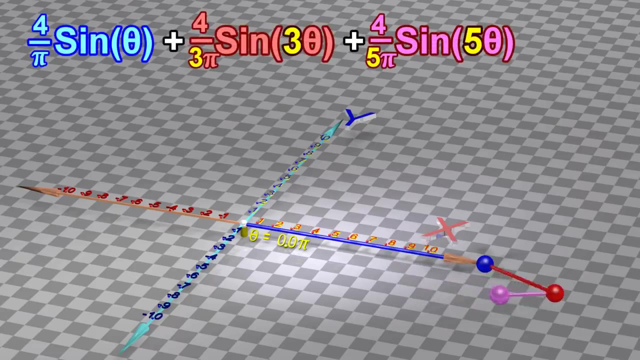 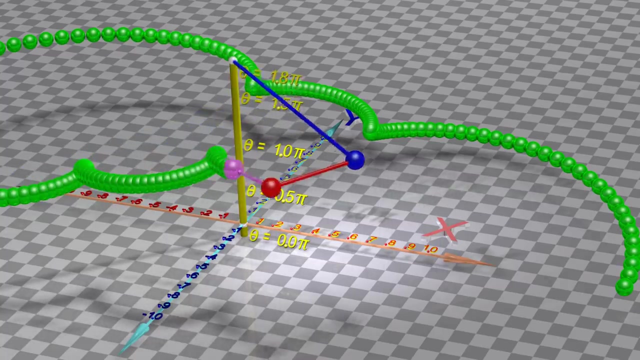 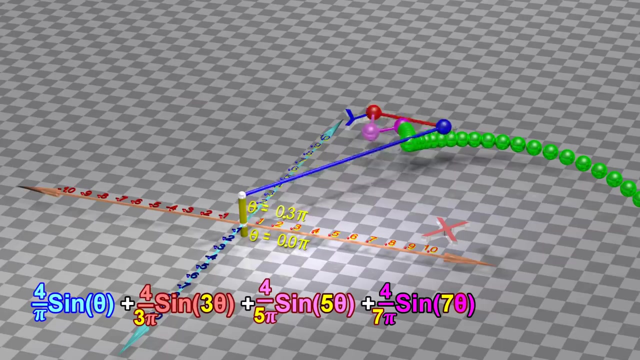 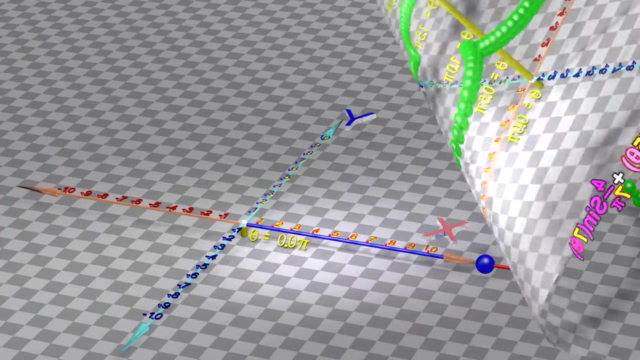 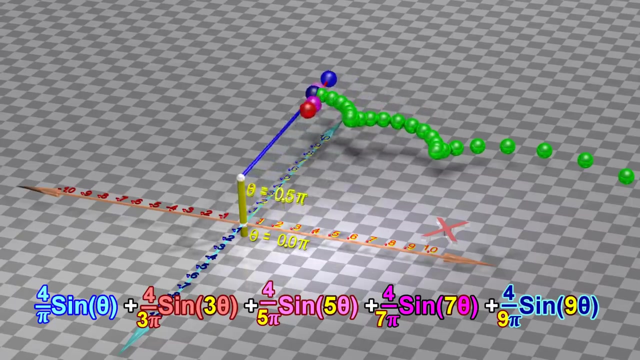 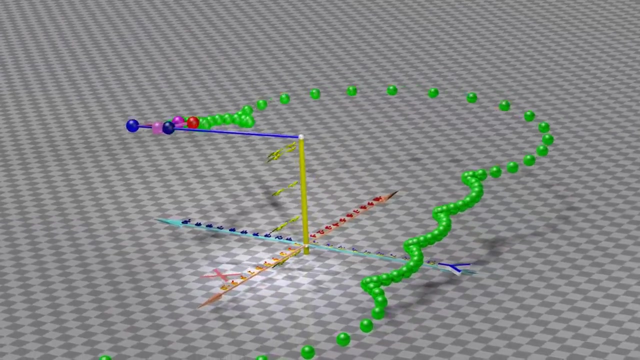 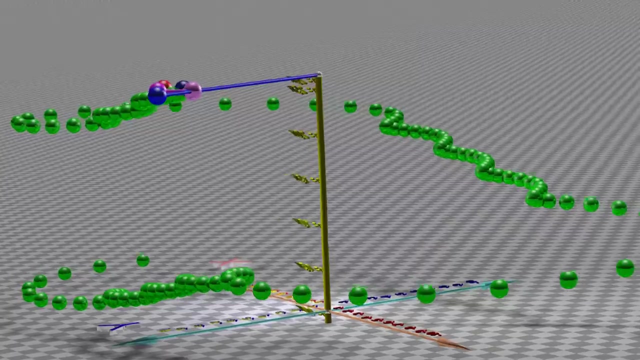 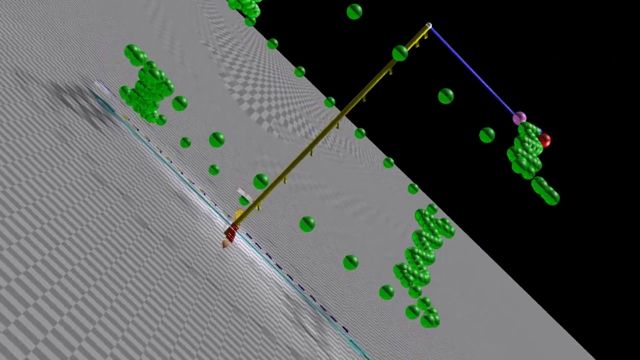 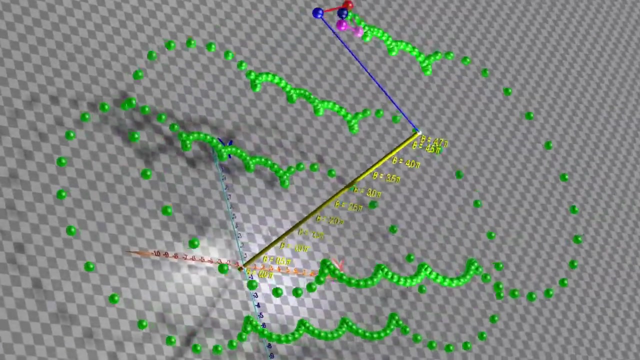 we can see that the nuros is solving the problem with a fraction of the normalre desen stumbled. We can add together three sine waves. We can add together four sine waves. We can add together five sine waves. © transcript: Emily Beynon. 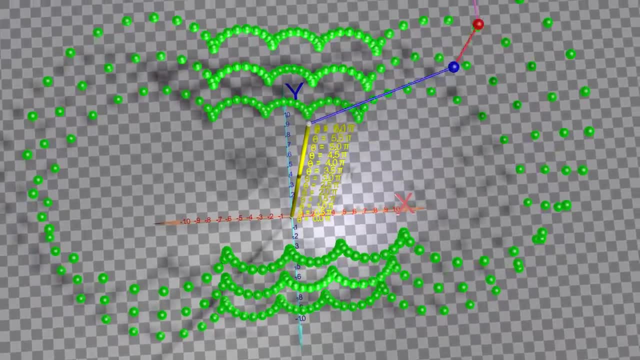 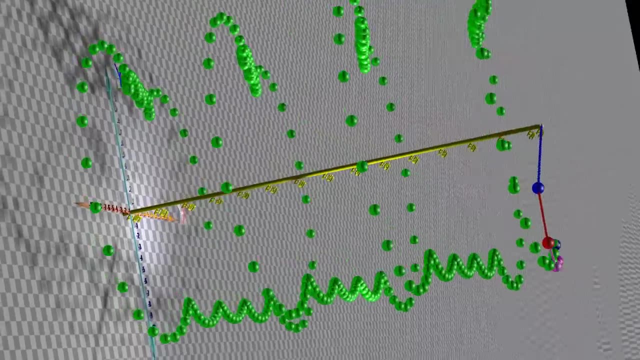 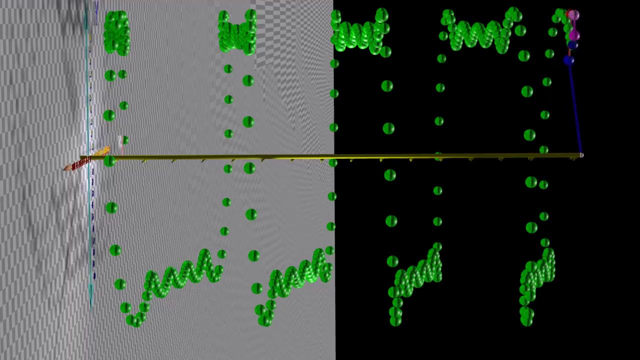 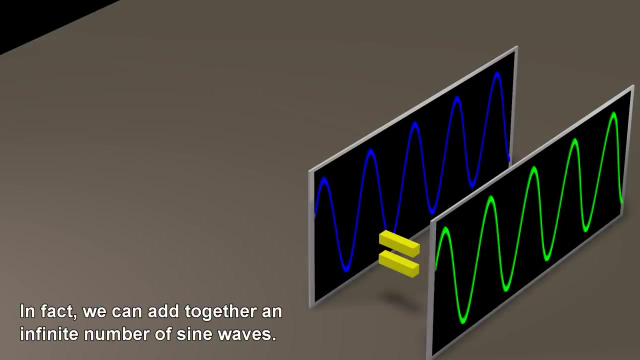 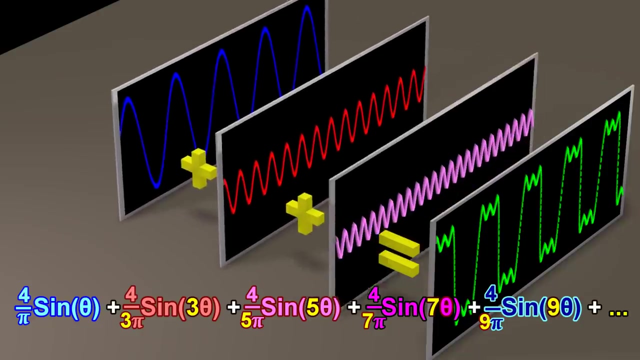 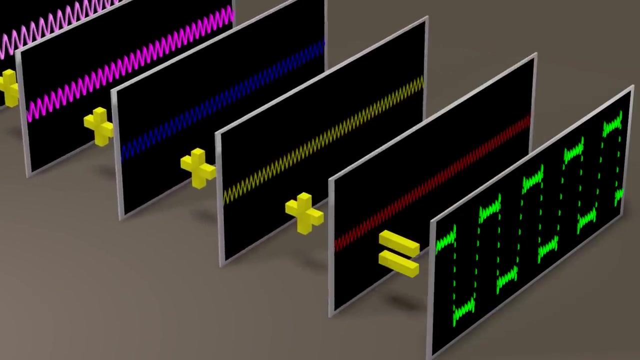 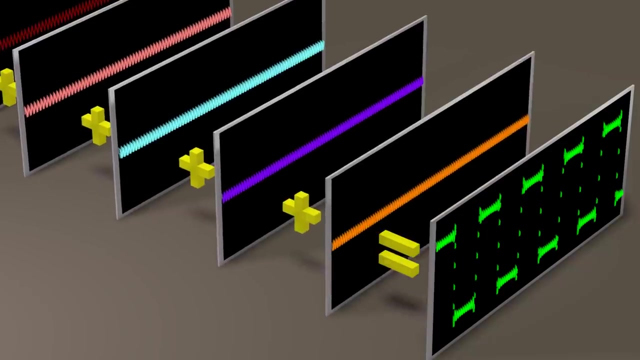 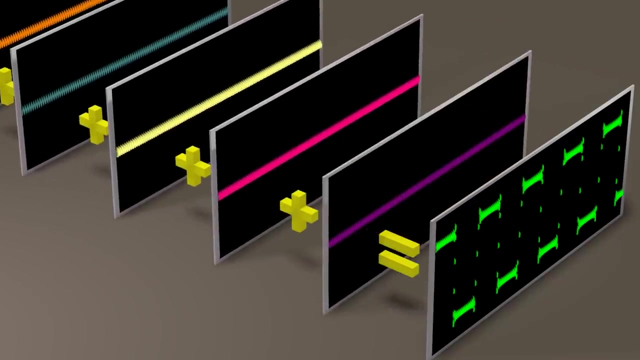 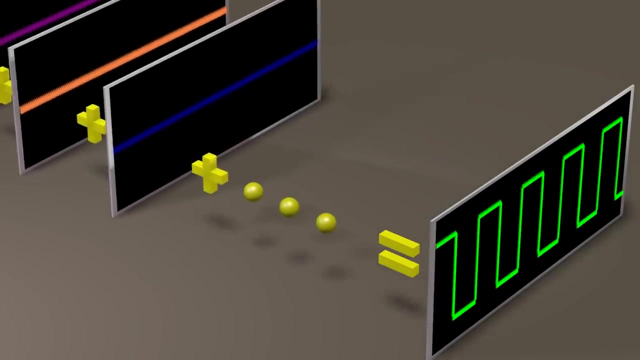 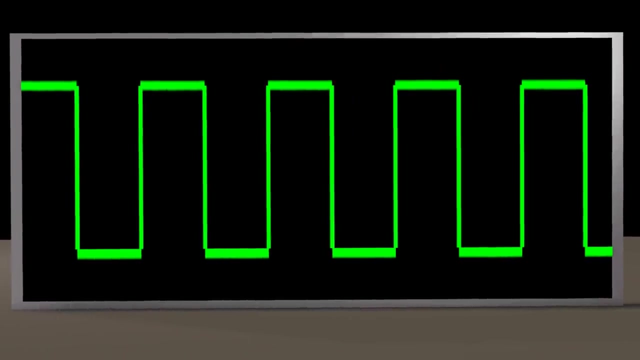 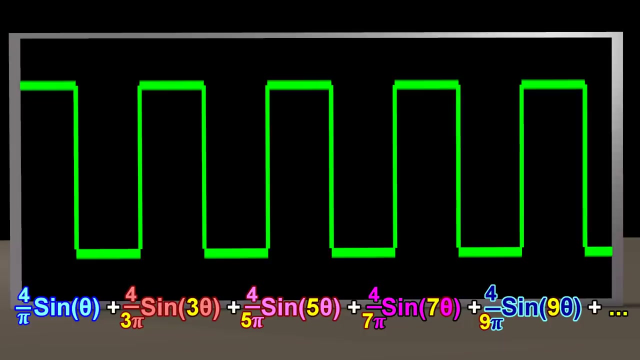 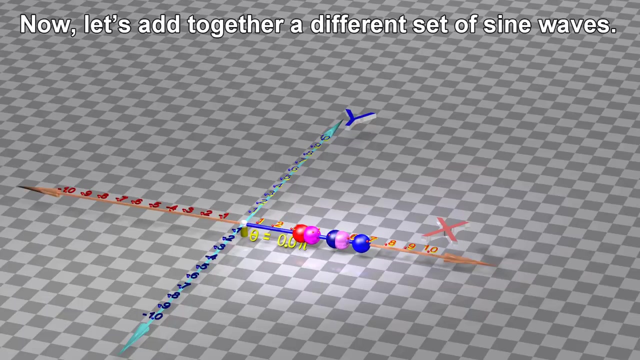 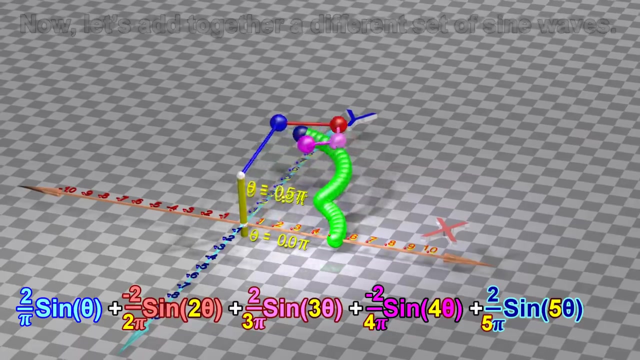 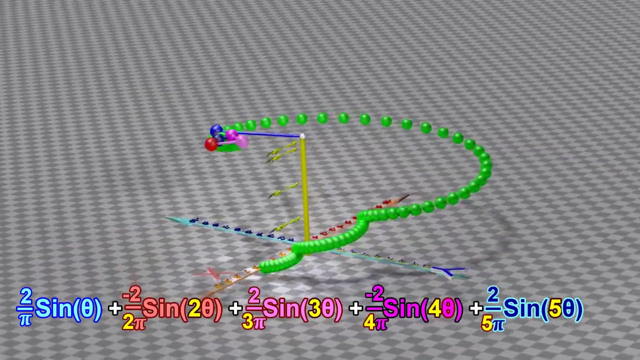 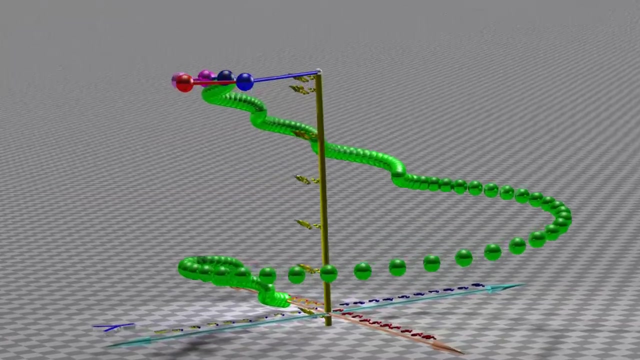 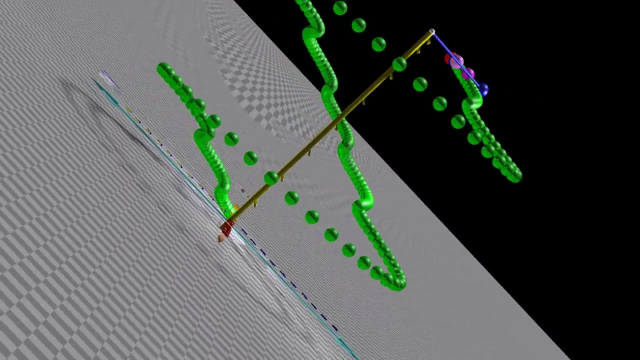 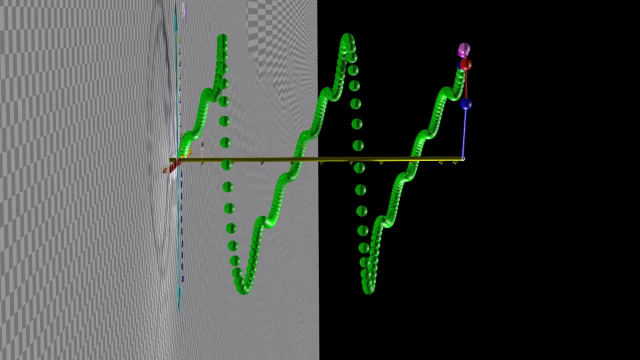 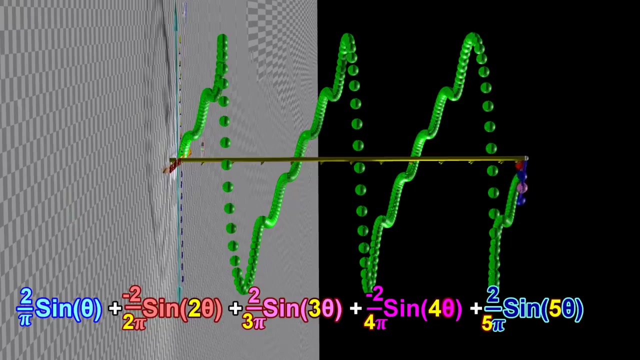 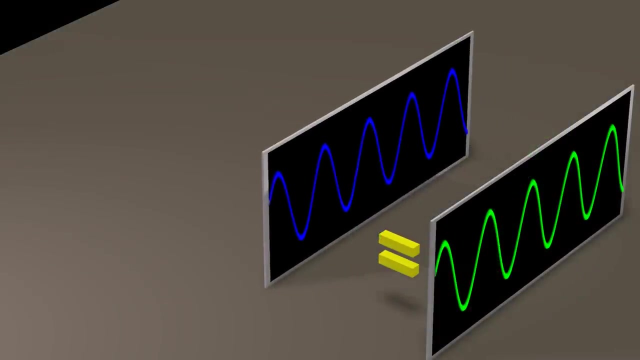 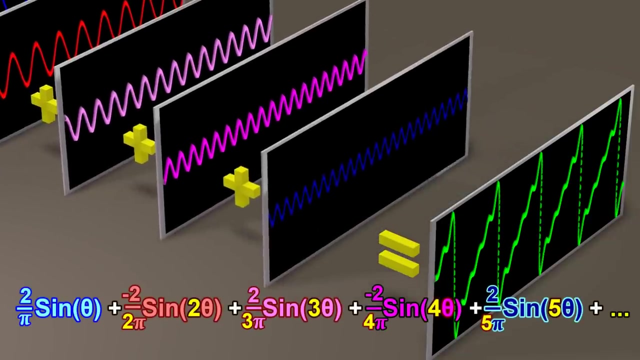 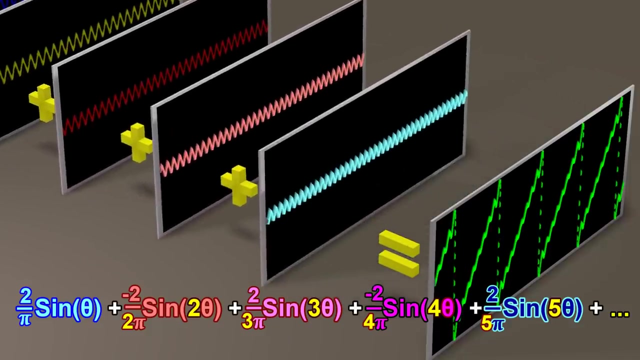 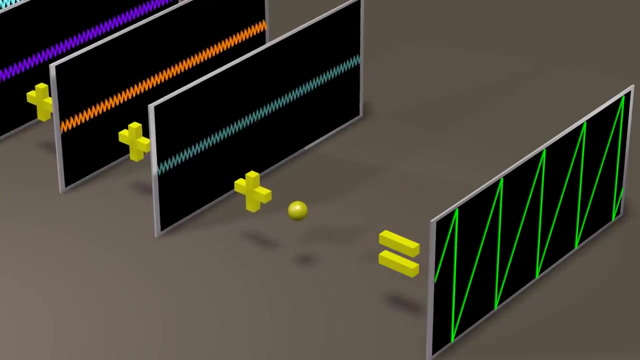 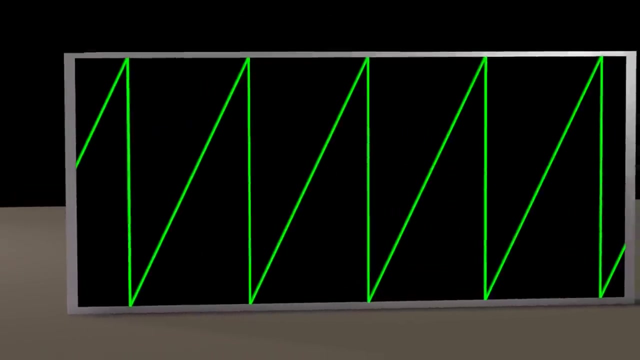 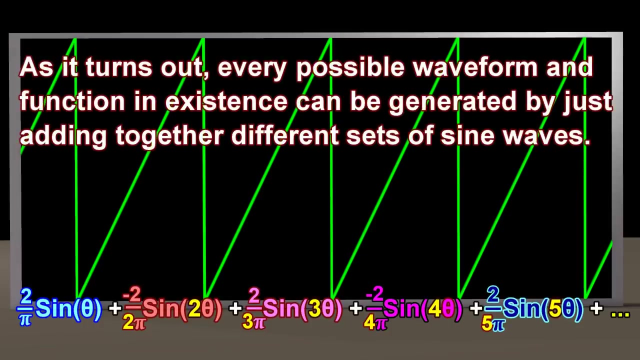 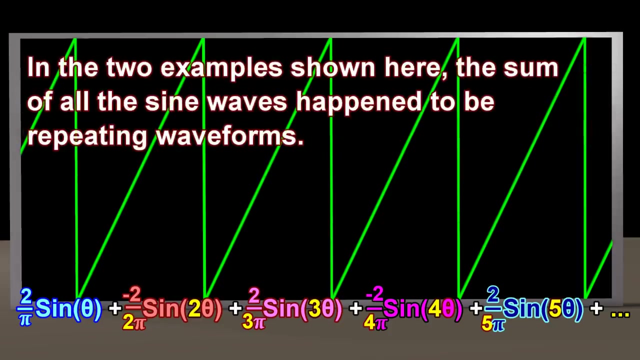 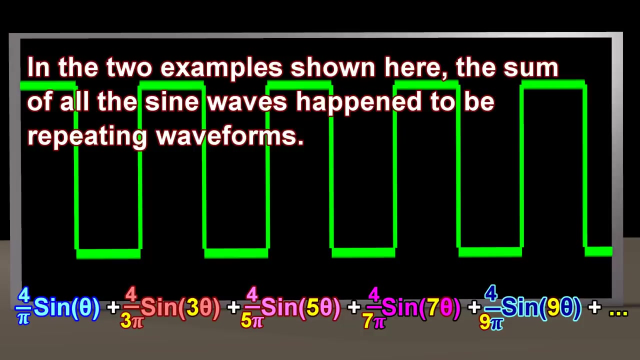 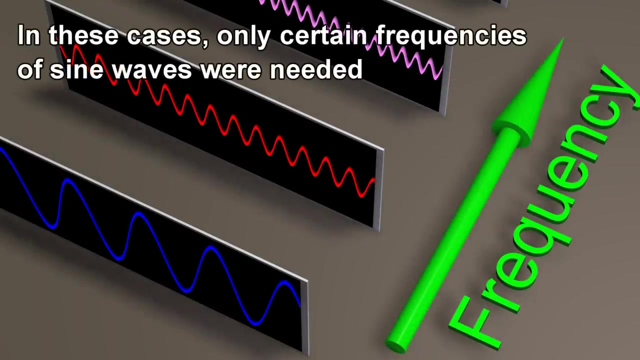 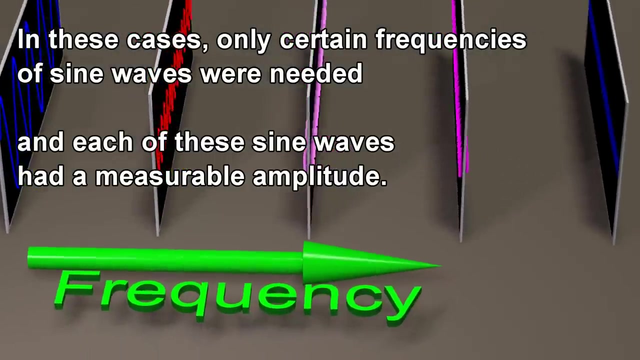 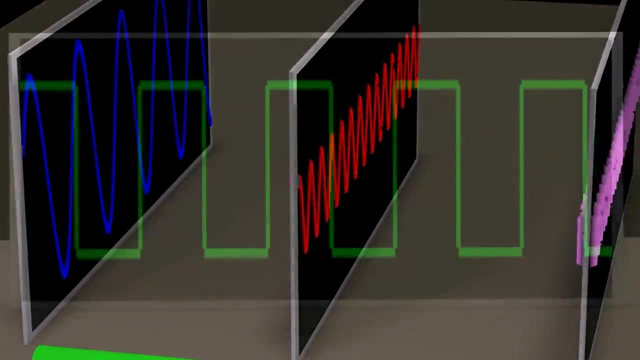 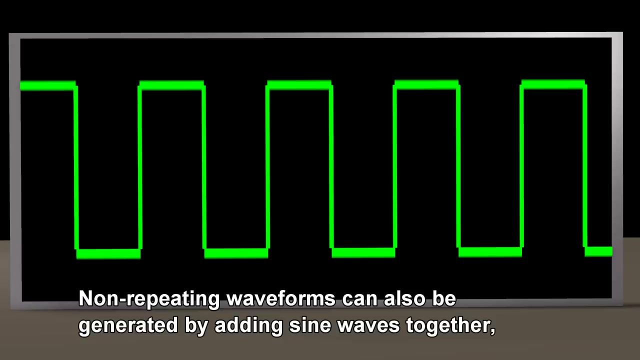 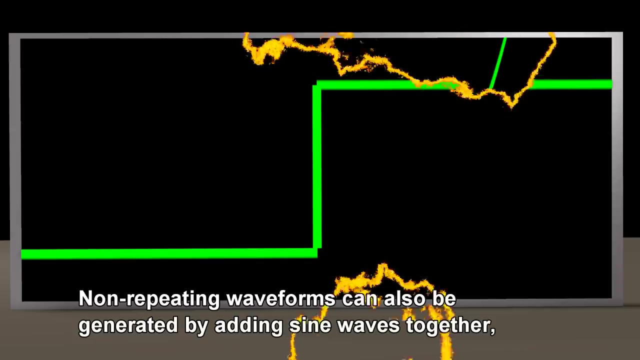 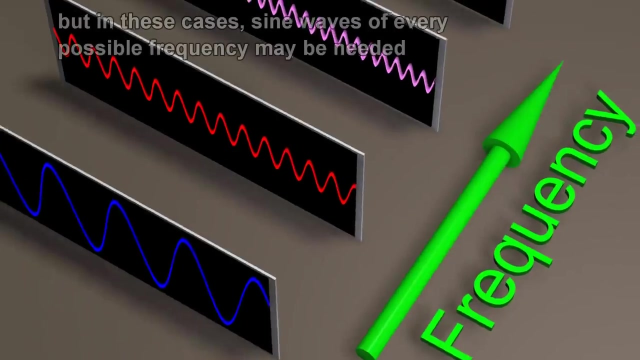 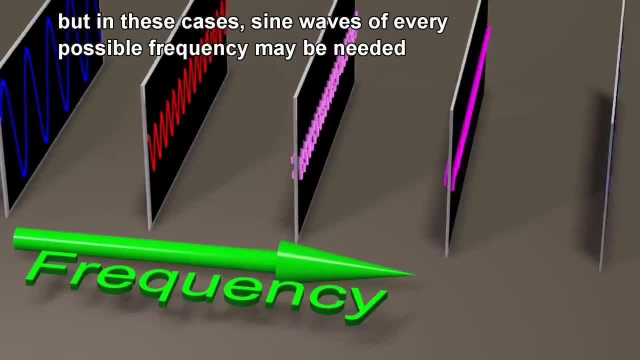 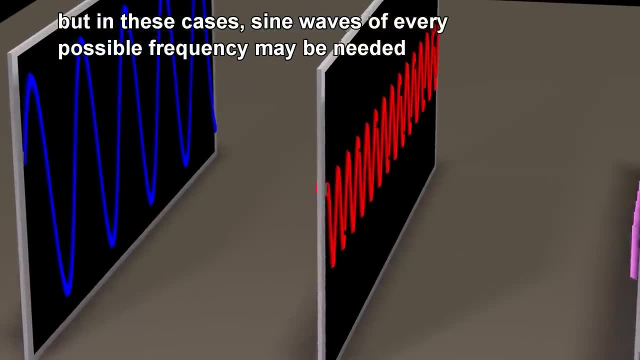 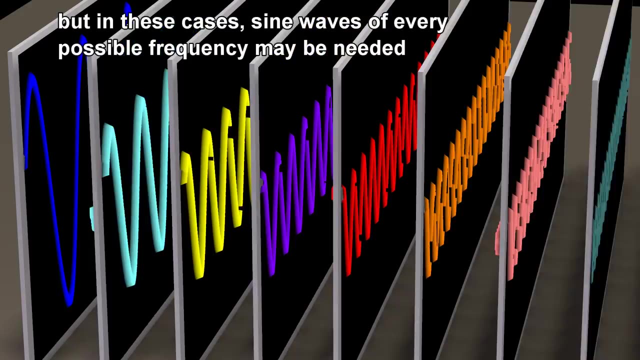 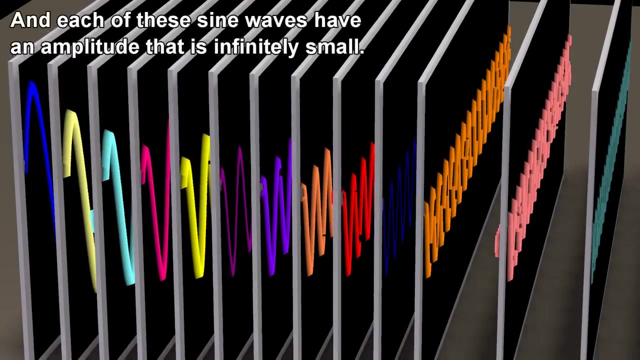 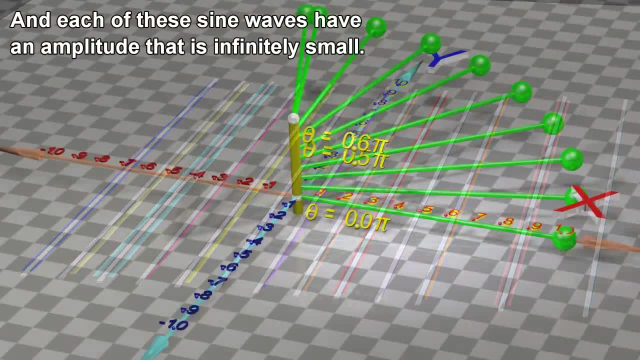 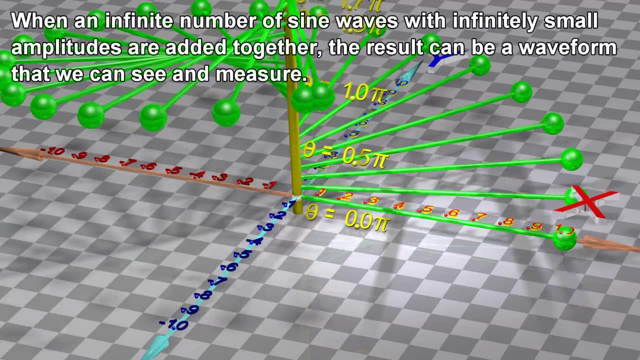 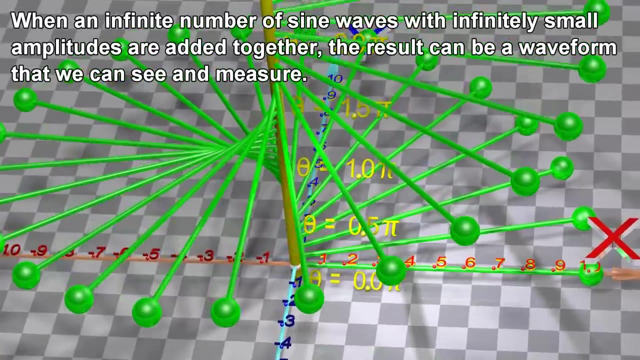 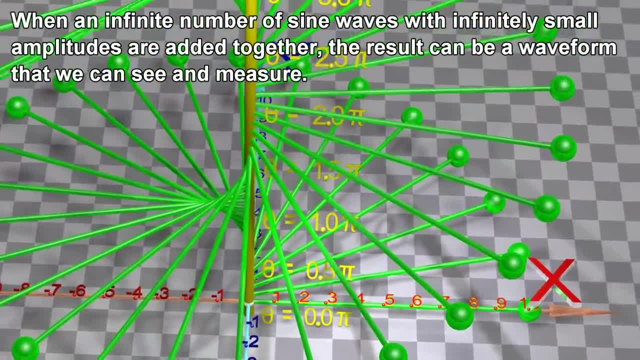 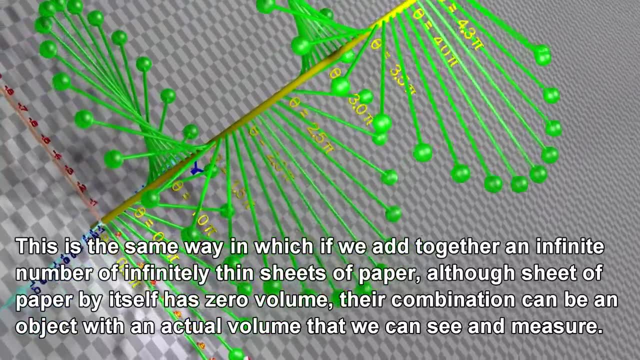 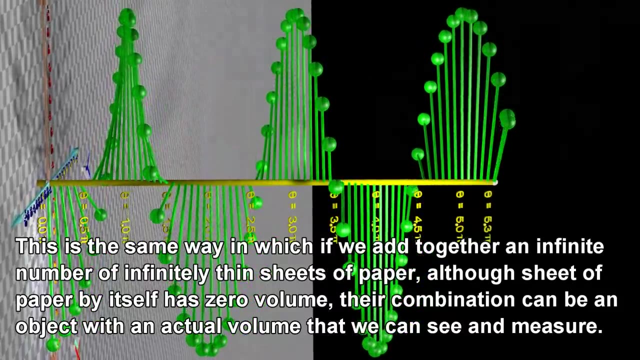 that we can see and measure. This is the same way in which, if we add together an infinite number of infinitely small amplitudes, we can see thin sheets of paper, Although each sheet of paper by itself has zero volume. their combination can be an object. 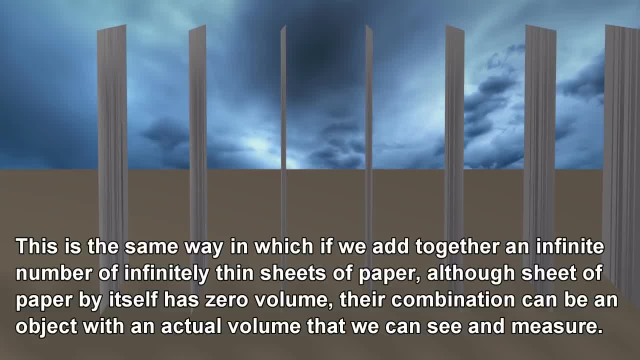 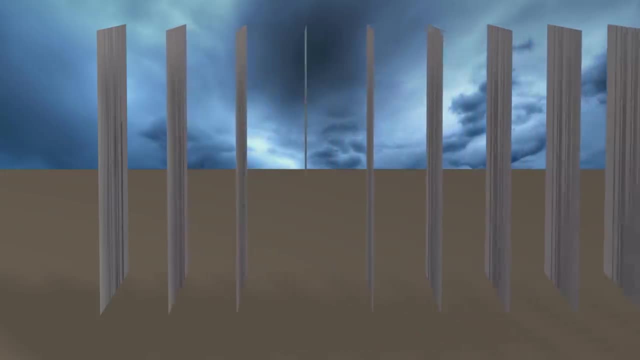 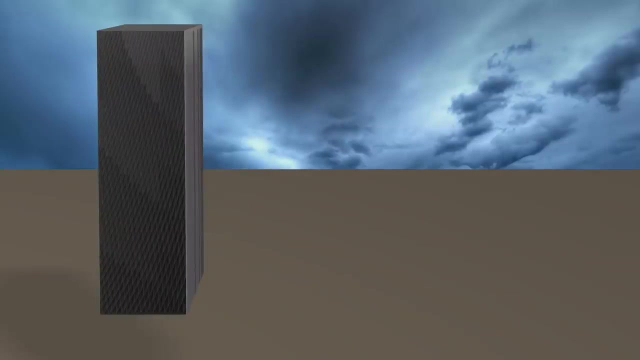 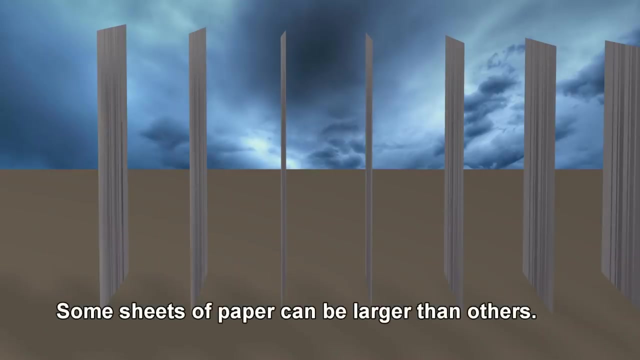 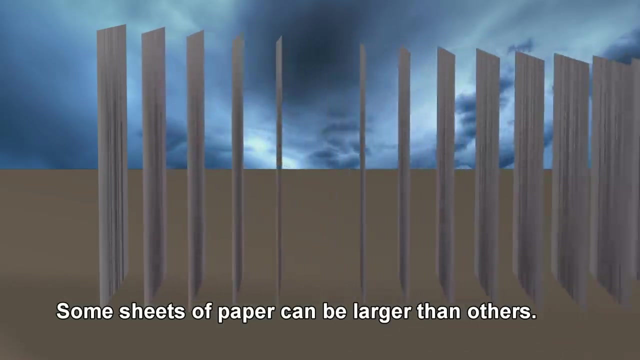 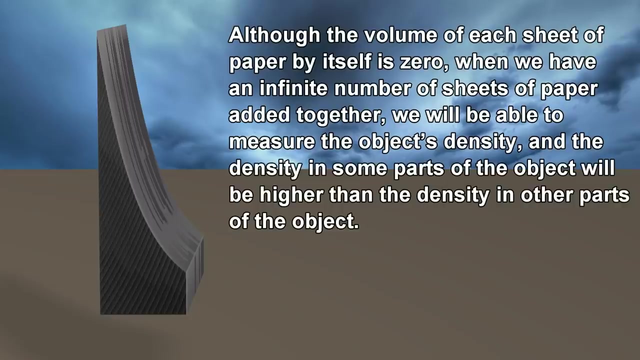 © transcript: Emily Beynon. Some sheets of paper can be larger than others. © transcript: Emily Beynon. © transcript Emily Beynon. © transcript: Emily Beynon. Although the volume of each sheet of paper by itself is zero, when we have an infinite number of sheets of paper added together, 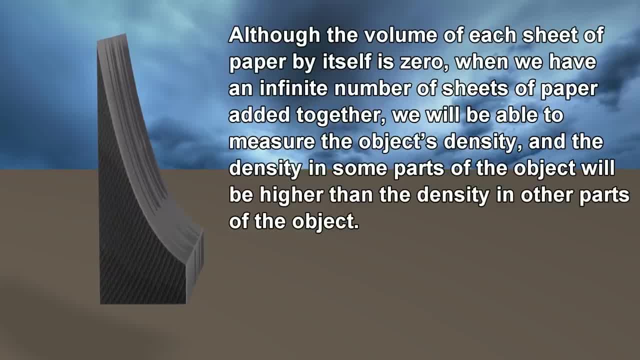 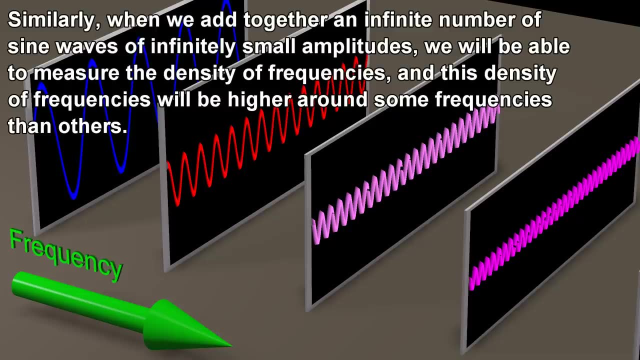 we will be able to measure the object's density, and the density in some parts of the object will be higher than the density in other parts of the object. Similarly, when we add together an infinite number of sine waves with infinitely small amplitudes, 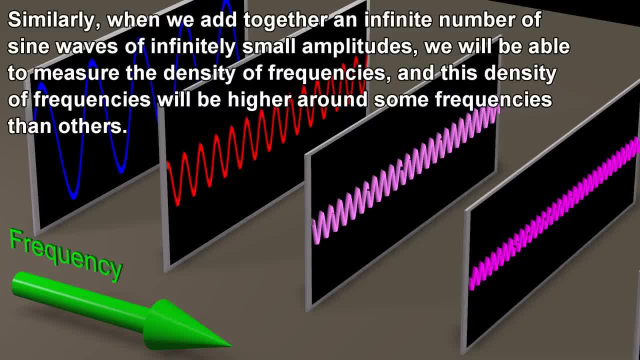 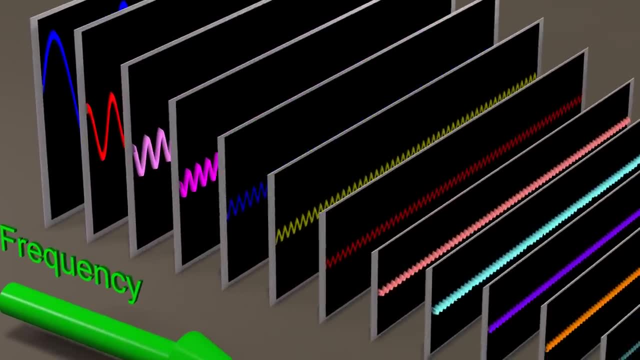 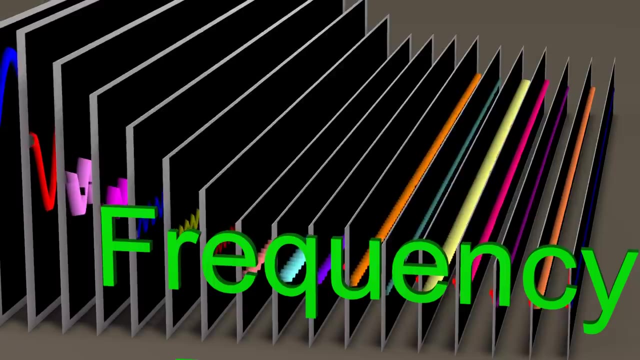 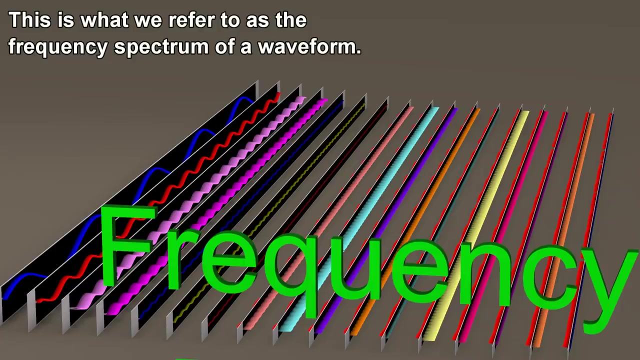 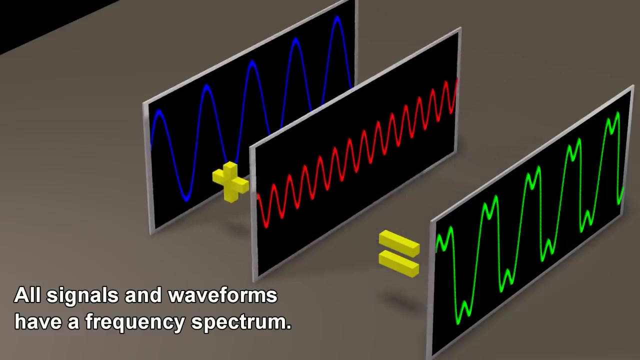 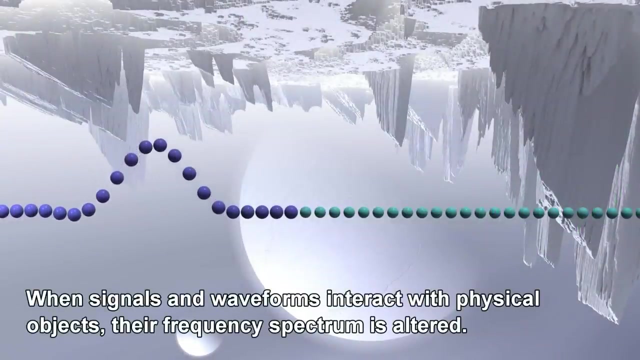 we will be able to measure the density of frequencies, and this density of frequencies will be higher around some frequencies than others. This is what we refer to as the frequency spectrum of a waveform. All signals and waveforms have a frequency spectrum When signals and waveforms interact with physical objects. 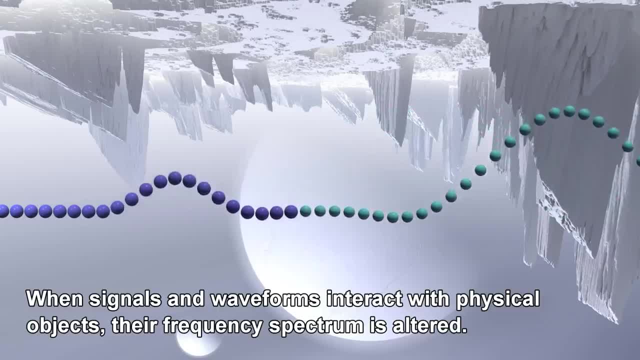 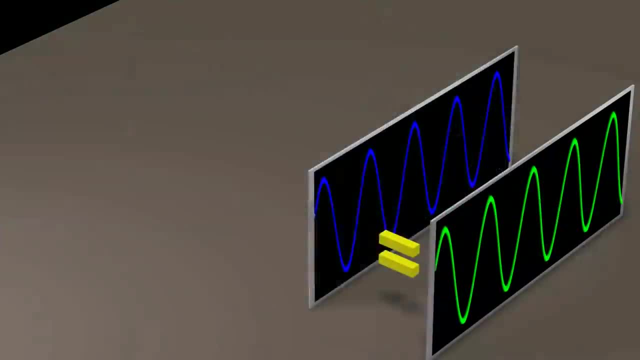 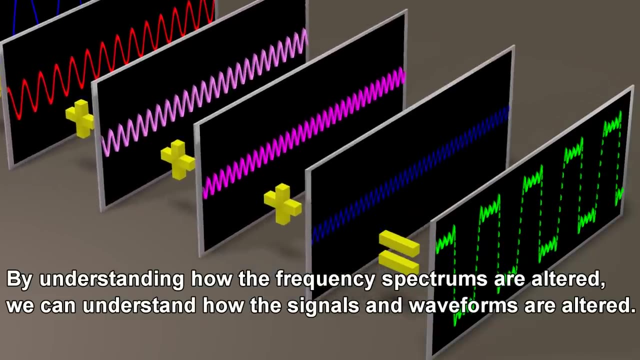 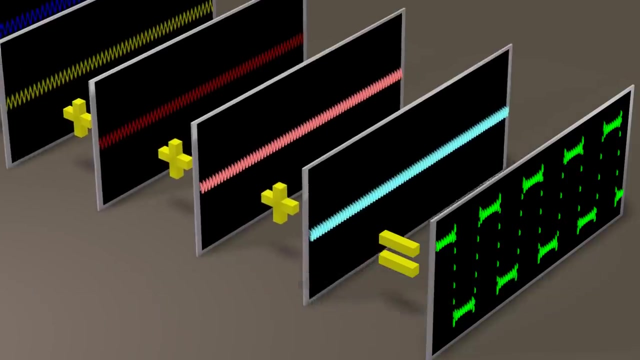 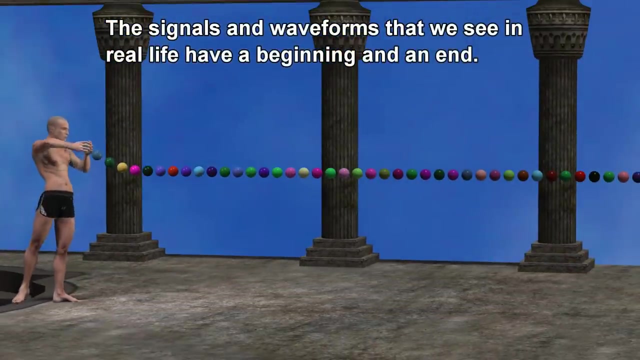 their frequency spectrum is different. The frequency spectrum is altered. By understanding how the frequency spectrums are altered, we can understand how the signals and waveforms are altered. The signals and waveforms that we see- we see in real life- have a beginning and an end. 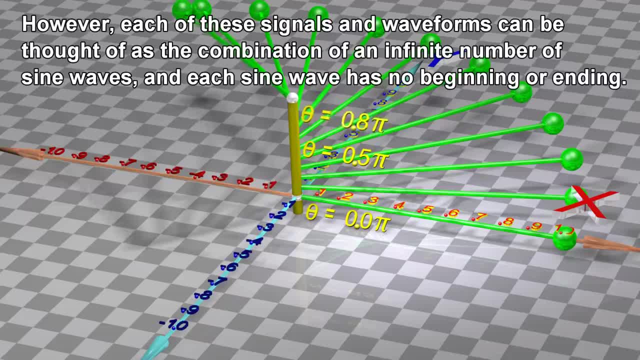 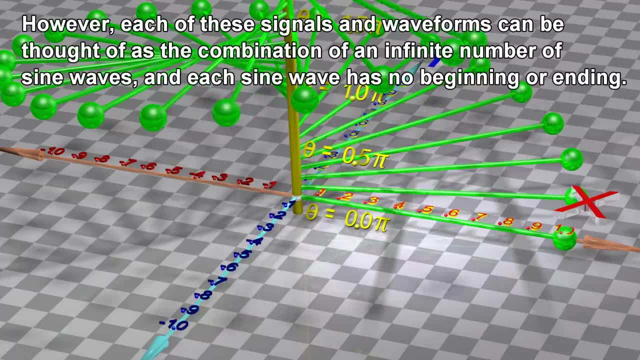 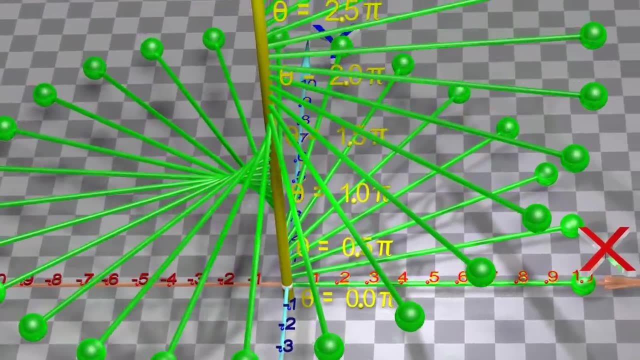 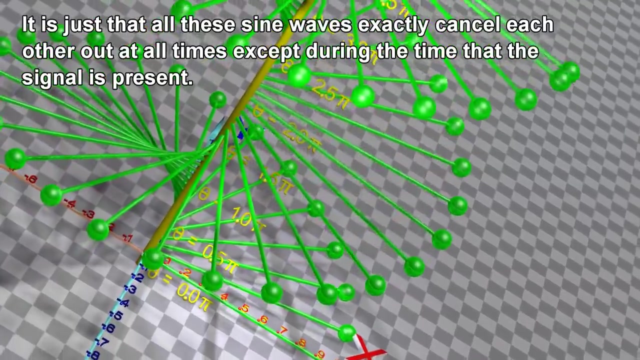 However, each of these signals and waveforms can be thought of as the combination of an infinite number of sine waves, And each sine wave has no beginning or ending. It is just that all these sine waves exactly cancel each other out at all times. 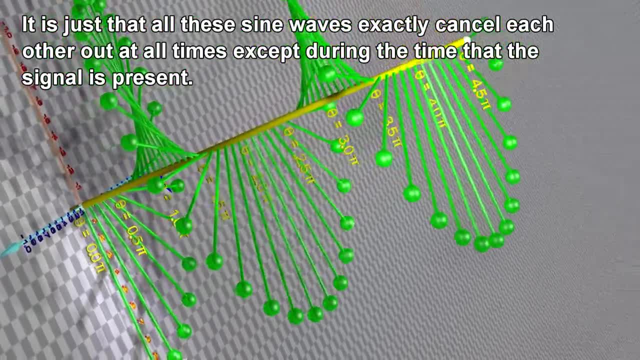 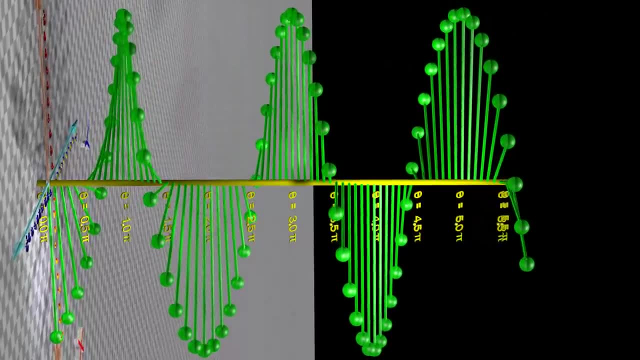 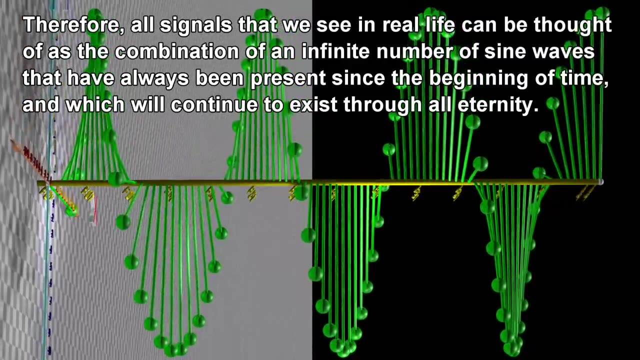 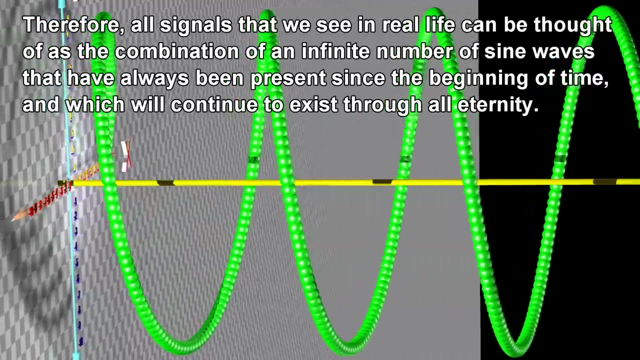 except during the time that the signal is present. Therefore, all signals that we see in real life can be thought of as the combination of an infinite number of sine waves that have always been present since the beginning of time and which will continue to exist through all eternity.